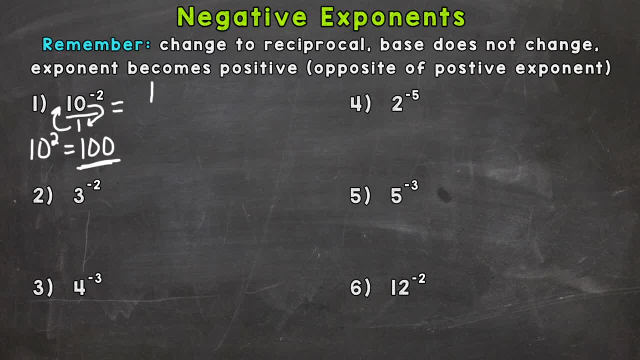 that we need to do this. So we now have a numerator of 1.. Our base of 10 stays the same And our exponent of negative 2 is now positive once it's changed to this reciprocal. So now we're able to solve and find our answer. So we know that 10 to the second power equals 10 times 10.. So our answer: 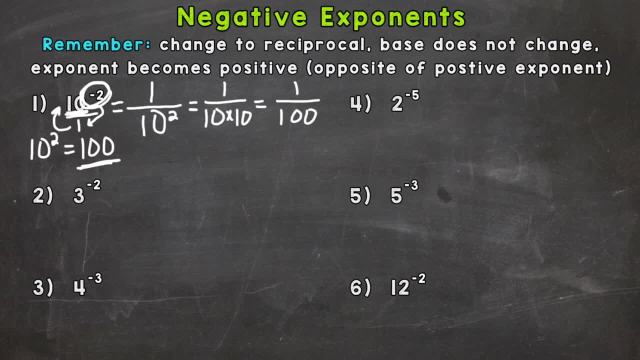 is going to be well. 10 times 10 equals 100.. Our answer is one hundredth. So you can see how these two are related when we have a positive or a negative exponent there. Again, positive exponent will increase the value of our base of 10, right, We went from 10. 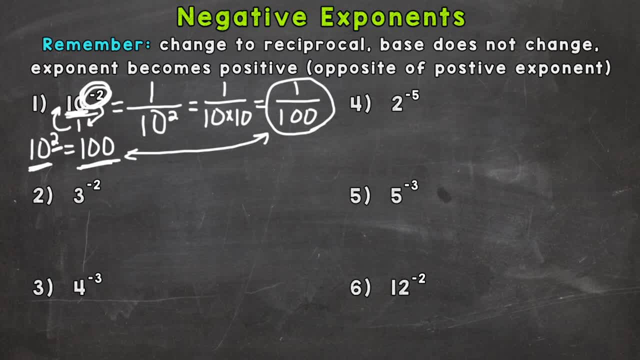 and we got it to equal 100. And negative exponent is going to decrease our value. right, We went from 10 and now we ended up with one hundredth, But we do not get a negative number. So let's take a look at number 2.. 3 to the power of negative 2.. So we need the reciprocal, So we can put 3. 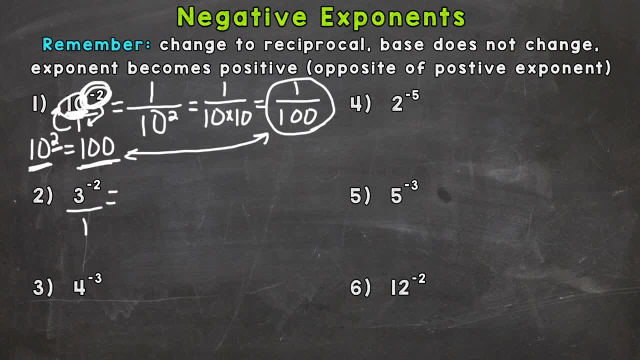 to the power of negative 2 over 1 to create a fraction, And it does not change the value of that 3 to the power of negative 2.. But when we solve it we need to change it to the reciprocal, which means flipping that fraction. So the 1 is now on top, Our base of 3 stays the same And this negative 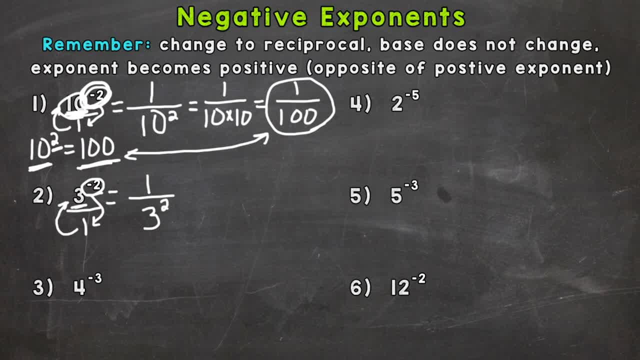 2 changes to a positive 2.. Now we can solve: And 3 to the power of 2 equals 9, right 3 times 3.. So our answer is one-ninth. Now let's take a look to see how that relates to 3, to the power of a positive 2.. And that: 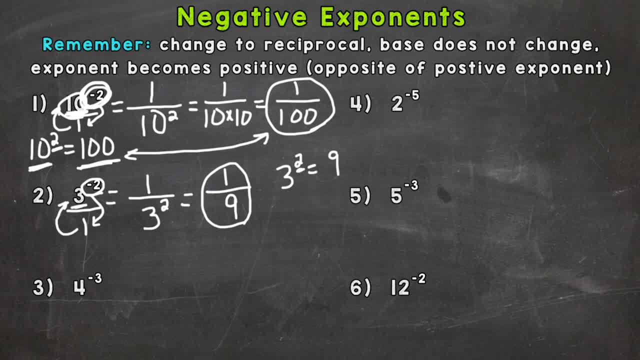 equals 9.. So the positive 2 gives us 9. And the negative 2 gives us one-ninth. Let's take a look at number 3.. So let's change to the reciprocal, which would be 1 over 4.. Or I'm.